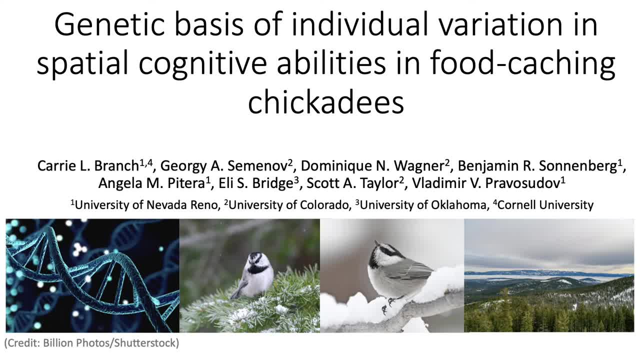 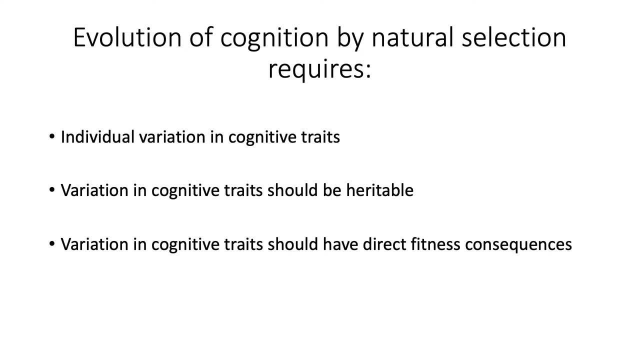 Today I'm going to talk about genetic bases of individual variation and spatial cognitive abilities in food caching chickadees, which is a big collaborative project with Dr Scott Taylor from the University of Colorado, Boulder, led by Carrie Branch. Understanding how cognitive abilities evolve remains one of the important questions in 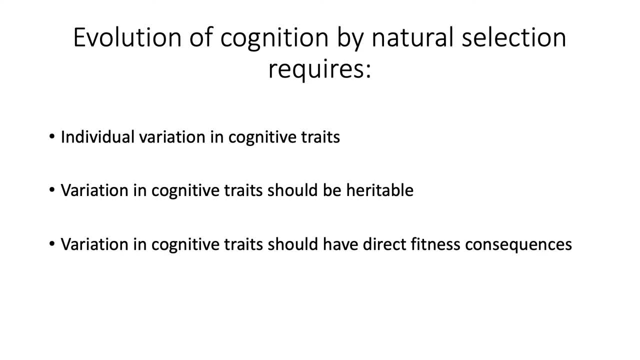 evolutionary biology, Animal exhibits large variation in cognitive abilities, both within and between species. but cognition also is a very flexible trait that may be affected by development, environment and individual experiences. At the same time, our understanding of heritability of cognitive traits under a genetic basis remains poor. For cognitive 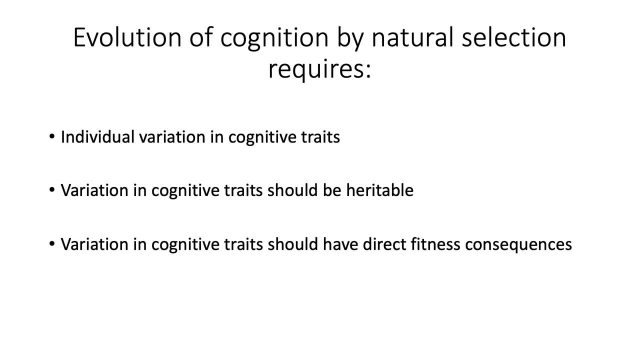 abilities to be affected by natural selection. we mainly need three conditions to be met: First, individual variation should exist, which is well documented. Second, such variation should be heritable, which is poorly known. And third, the variation should have fitness. 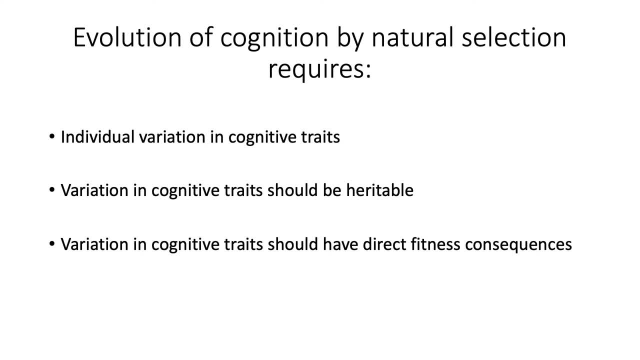 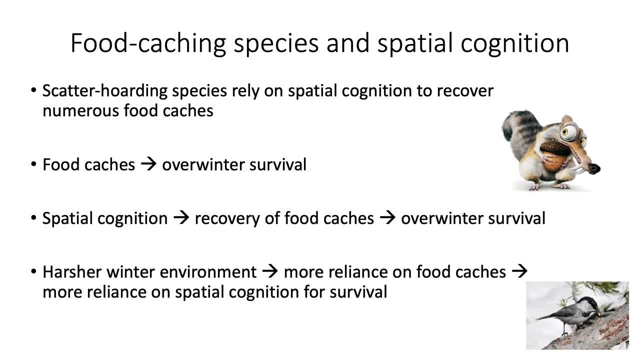 consequences also poorly known at this point. Food caching speed species present a great system to investigate evolution of cognition and, more specifically, spatial cognition. Skitter hoarding species rely on spatial cognition to recover numerous food caches, and we're talking about tens of thousands and hundreds of thousands of. 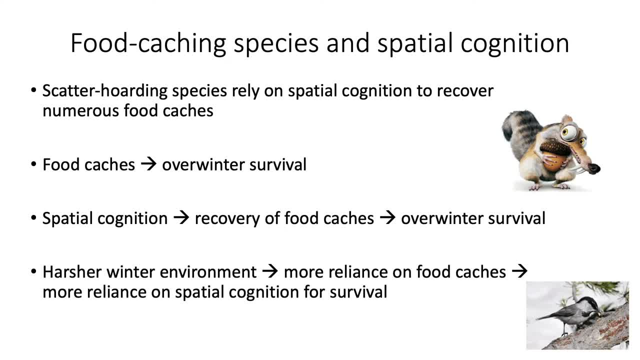 scattered food caches. Food caches are critical for winter survival. Not being able to access their food caches will result in mortality. Spatial cognition is necessary for recovery of food caches and hence it is necessary for overwinter survival. So our main hypothesis that we've been working on for a long time: 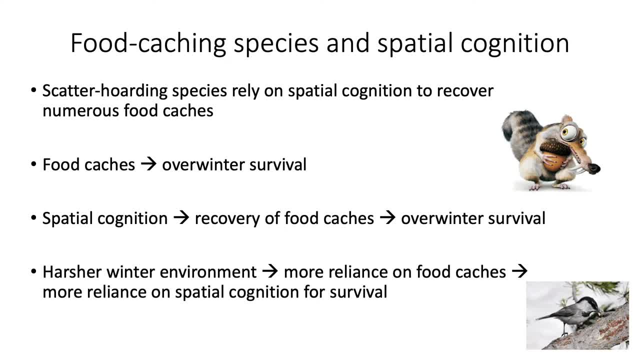 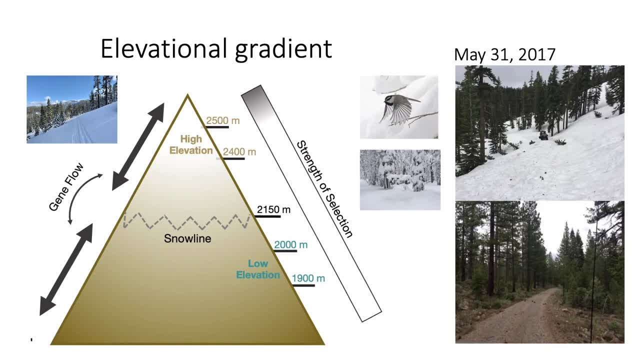 now is that harsher winter environment should lead to more reliance on food caches and hence it should lead to more reliance on spatial cognition for survival. After showing that winter environment is indeed associated with differences in spatial cognition and hippocampal morphology in black-capped chickadees on a continental scale, our work 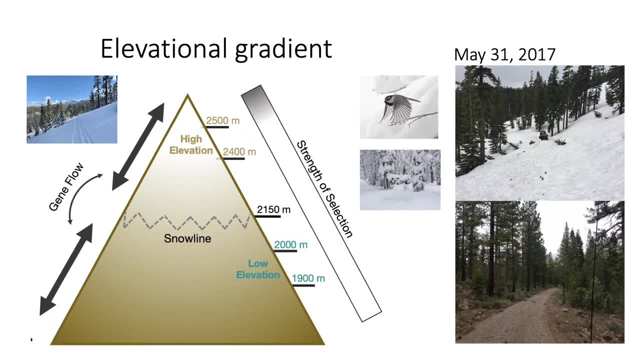 was focused on investigating winter climate and spatial cognition on a small spatial scale along an elevation gradient in Mt Jackson. Winter conditions change drastically along an elevation gradient, but such differences are not gradual. The biggest changes occur above the snow line, The snow line which 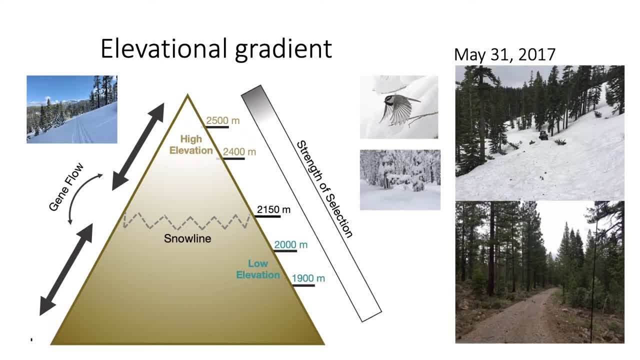 varies in elevation between mountain ranges indicates elevation above which most winter precipitation comes as snow and below as rain. But, most importantly, the strength and severity of snowstorms are much higher above the snow line, resulting in rather harsh winter conditions for the chickadees. On the right you can see conditions at high elevation, the top. 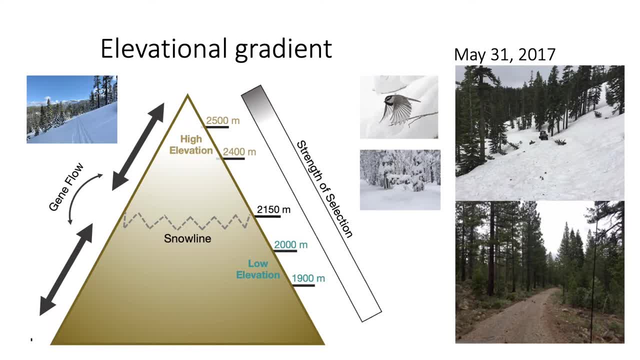 photo And low elevation at the bottom photo. on the same day, May 31, 2017, almost 6 feet of snow depth at high elevation. still, While there is some gene flow between elevations, chickadees are highly resonant and we have not documented a single bird that hatched at one elevation. 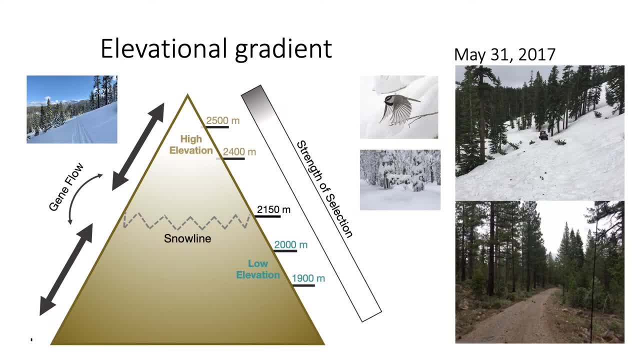 and bred at a different elevation, despite banning thousands of nestlings over the last eight years. Giving such drastic changes in winter conditions above the snow line, we expect the strength of selection on spatial cognition needed to recover caches to be stronger above the snow line, as caches are likely to be much more critical for winter survival. 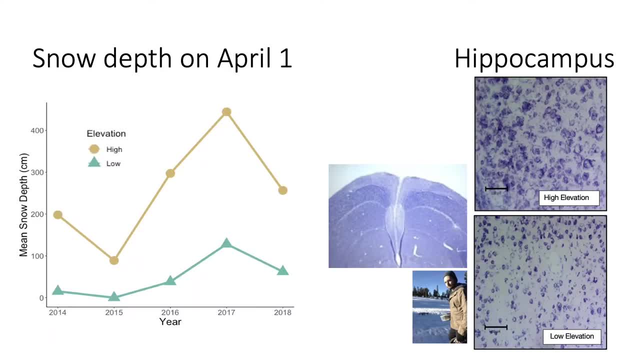 at high elevation. A comparison of chickadees from high and low elevation in the lab done by Cody Fries, who was a master's student in my lab, indeed documented significant differences both in spatial learning and memory and in the hippocampus morphology between high and low elevation. On the picture: 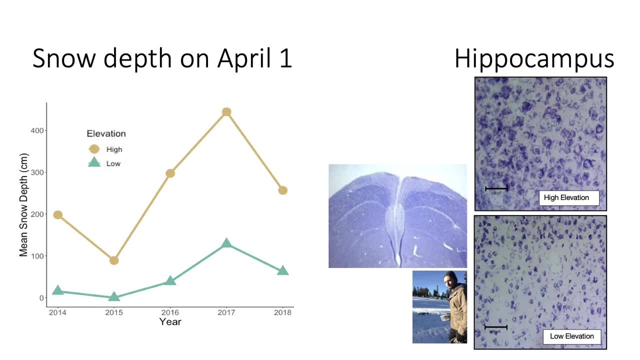 on the right you can see a picture of neurons at high elevation and low elevation and you should be able to see easily that there are way more neurons and there are bigger neurons at high elevation. Following our comparative lab-based studies, we have established a novel RFID-based system. 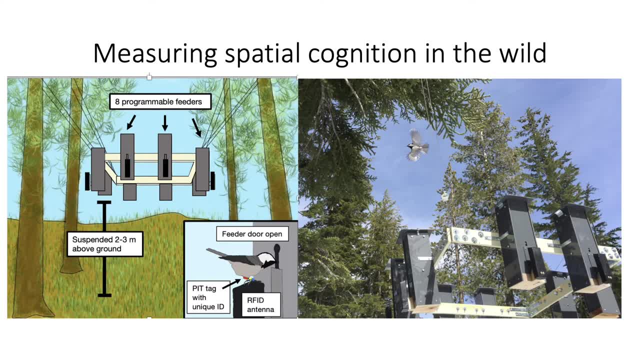 of measuring spatial learning and memory abilities in wild chickadees in their natural environment. We use a radial maze analog with eight feeders positioned equidistantly on a square frame suspended above the ground. We program RFID feeders so that each bird has to learn spatial. 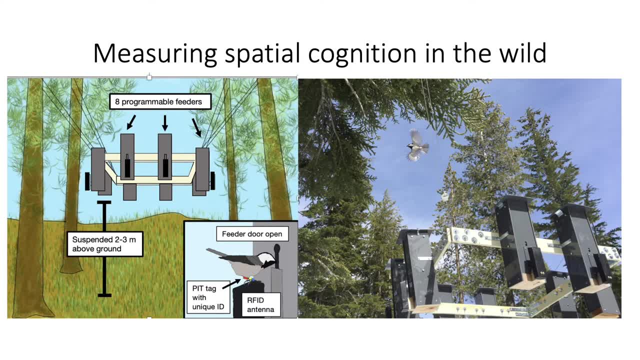 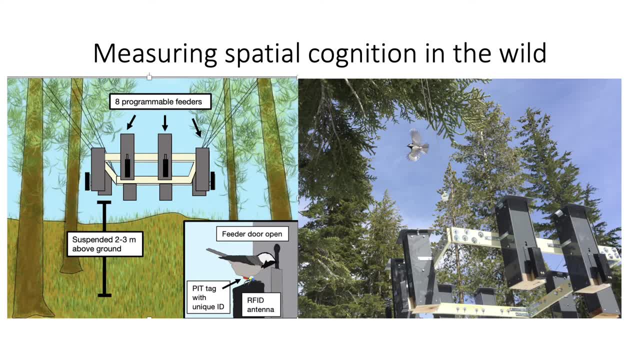 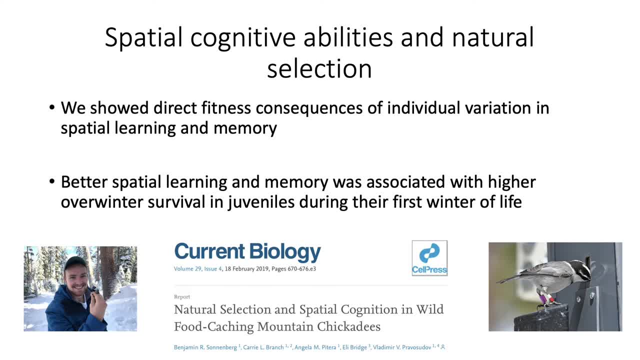 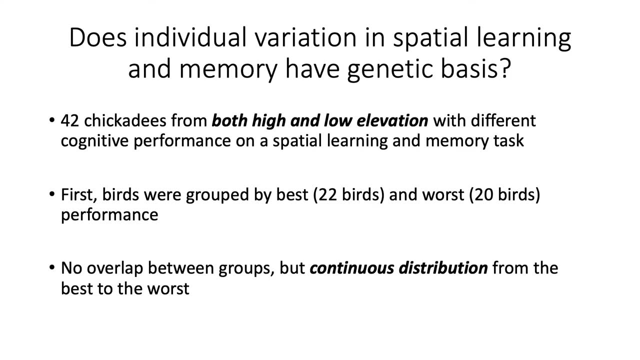 spatial learning and memory in mountain chickadees is indeed under natural selection, as in juvenile birds in their first winter, variation in spatial learning and memory abilities was associated with differences in overwinter survival. Only the juveniles with better spatial cognition survived their first winter. A critical question now is whether individual variation in spatial cognitive 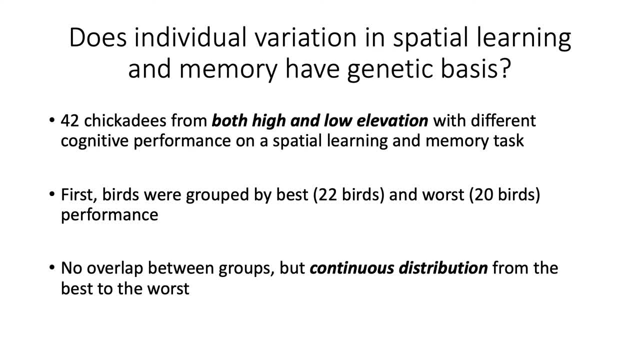 abilities is heritable and has genetic basis. To address this question, we selected 42 chickadees from both high and low elevation, based on their cognitive performance. We selected the best birds at both high and low elevation and not so good birds from both high and low elevation, While 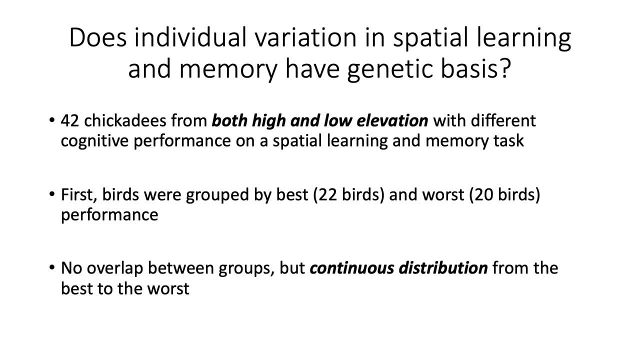 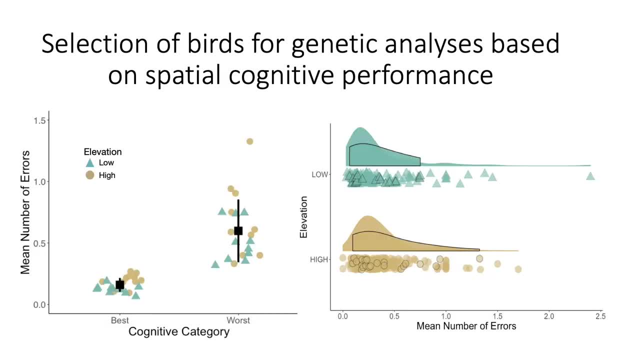 there was no overlap between the groups. there's continuous distribution connecting these two groups, rather than all birds in each group having identical performance. On this graph, you can see the distribution of selected birds based on their cognitive performance. On the left and on the right you can see how these selected birds fit into the overall distribution. 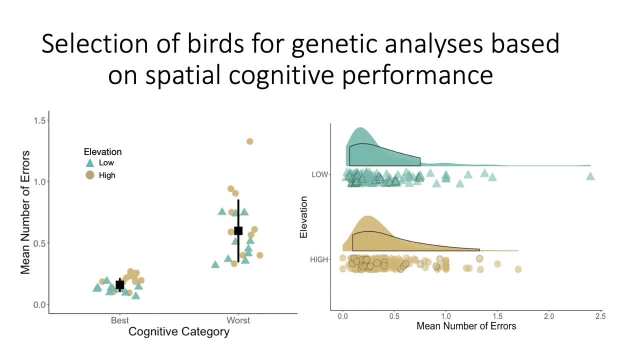 of all birds that we have tested. The selected birds have black outline and their symbols. The key thing here is also that you can see that the birds with not so good performance were not just some outliers, but they actually were representative of a pretty large part of the 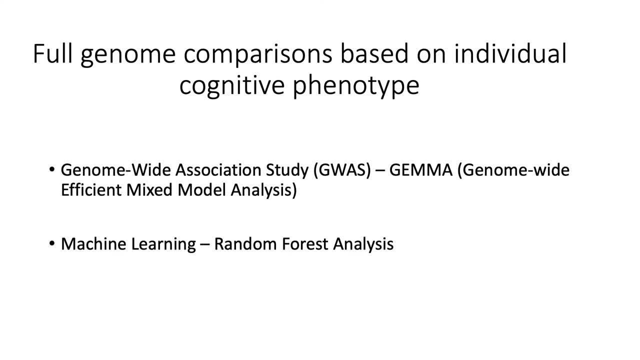 natural distribution. We have sequenced full genomes of these birds and align them to the reference genome of the black-capped chickadee. We use two methods to look for potential differences in genomes based on individual variation and spatial cognitive abilities. First, we use the genome-wide association analysis, GWAS. 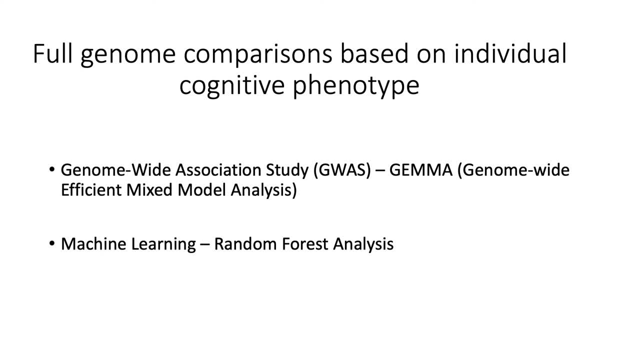 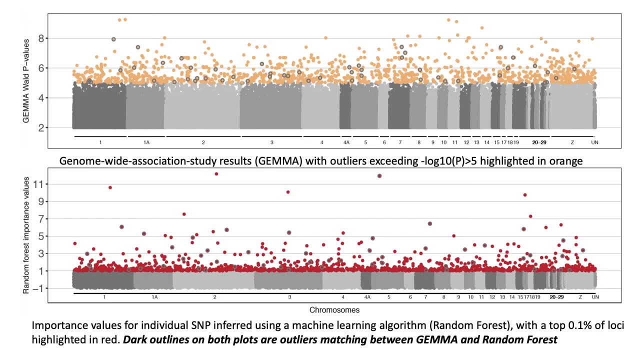 by using GEMMA, genome-wide efficient mixed model analysis, and second, we also used a machine learning approach using random force analysis. Both analysis identified many significant differences associated with variation in cognitive phenotype. as you can see on these graphs, The top graph shows results of the GEMMA or GWAS analysis and the bottom graph shows results of the machine learning. 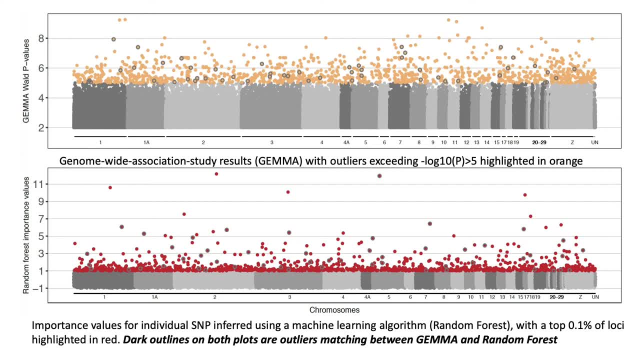 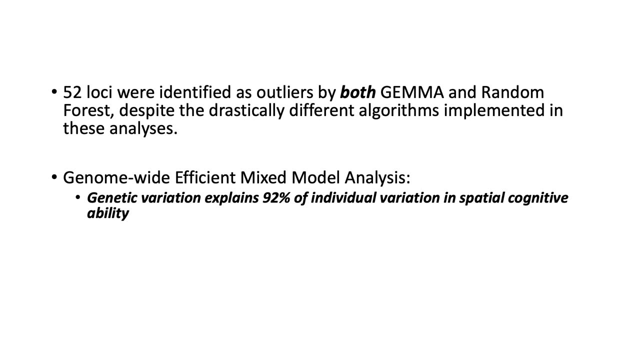 random force analysis. On both graphs, the black or gray outline of the symbols indicates the outliers picked by both analysis simultaneously. Overall, 52 loci were identified as outliers by both GEMMA and random force. despite the drastically different algorithms implemented on those different analysis, The most important thing is that genome-wide, efficient mixed model analysis. 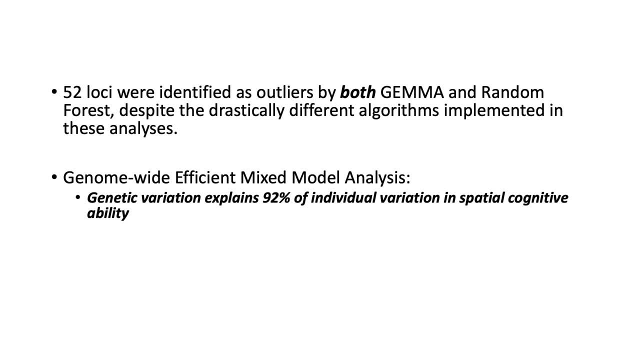 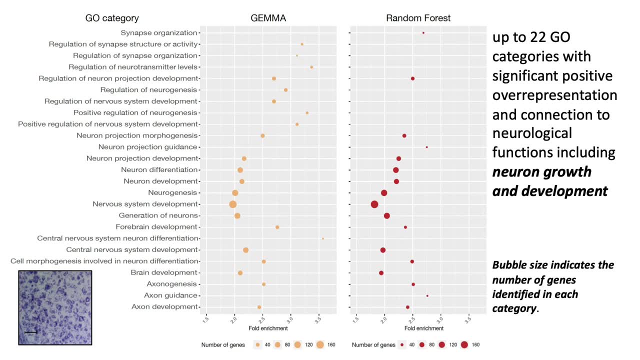 showed that genetic variation explained 92% of individual variation on spatial cognitive ability. Where are these differences in genome located? The GOA analysis identified up to 22 categories with significant over-representation and connections specifically to neurological functions, including neuron growth and development. What is striking here is that the distribution of